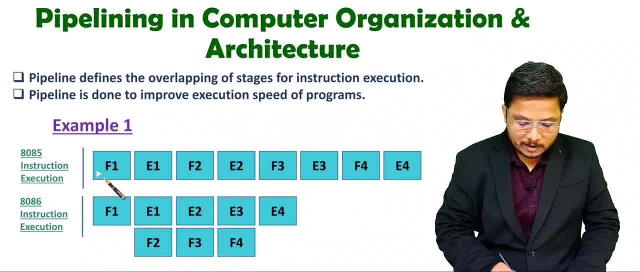 execution of instruction 1.. So, if you observe, sequential execution of instruction is happening over here. F1- E1 means execution of first instruction, as per fetch 1- execute 1.. Then F2- E2 means execution of second instruction, as per fetch 2- execute 2.. F3- E3 means execution of third instruction, and F4- E4 means execution of fourth instruction. Now, same execution that is been done in 8086 but along with 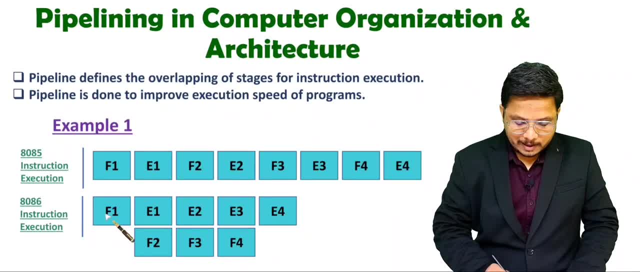 two stage pipelining. Here. if you observe, this execution is happening in parallel. How you see, first it is fetching first instruction and in second cycle, when it is executing first instruction, in parallel with that it is fetching second instruction. So in next cycle, what it does, it will execute second instruction and in parallel with that it will be fetching third instruction. and in next cycle it will be executing third instruction and in parallel with that it will fetch fourth instruction. 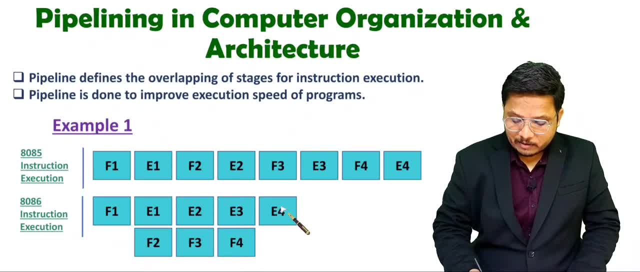 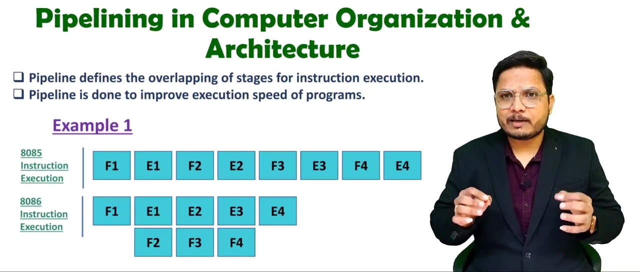 And in next cycle it will be executing fourth instruction, Right? So if you observe over here with 8086 because of two stage pipelining, you will be observing execution speed of program that is increasing very fast, Right? You can say almost two times execution speed is there in terms of pipelining over here, Right Here. my dear students, what is the basic concept that engineers have applied over here Previously? what was happening was like in CPU. 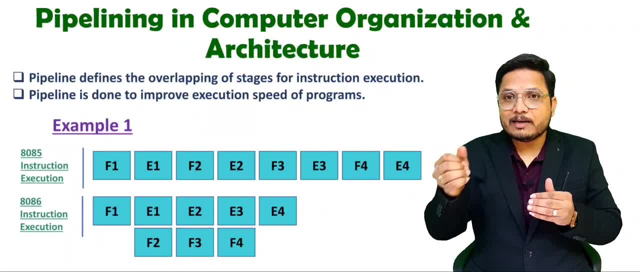 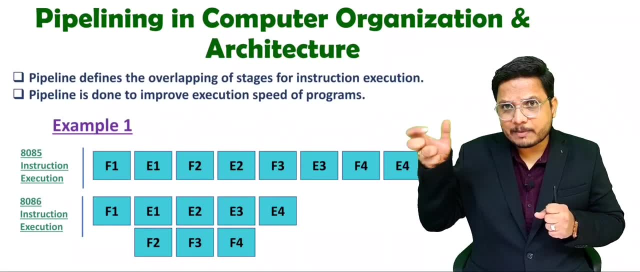 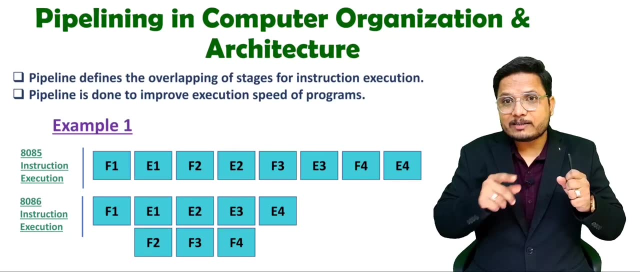 There was fetch After fetch, they were been decoding it. After decode, they were been executing it. But here, if you observe, when fetch is happening after that, when decode is happening, at that time, unit of fetch that is free, And when that decoded instruction that is getting executed, at that time, decode as well as fetch units are free. So instead of having all those units free, what they have done is they have make it active. How? 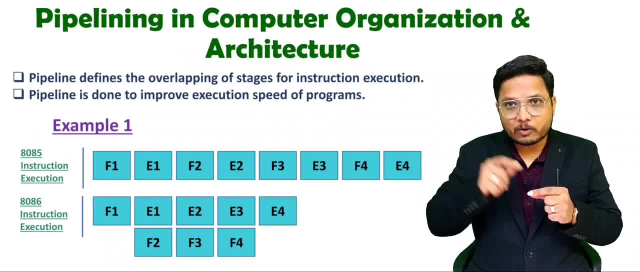 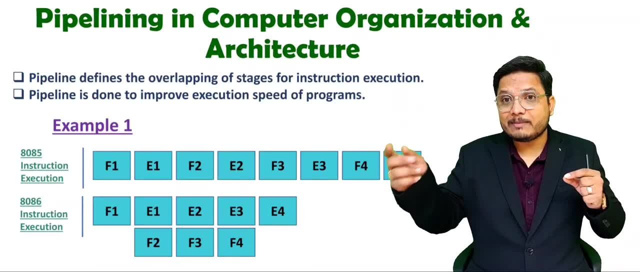 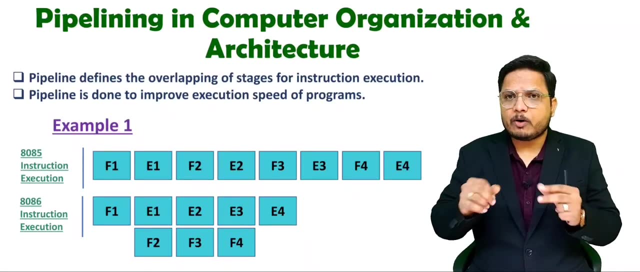 When first instruction is getting fetched, it will go into decode stage. When first is getting decoded, at that time second is getting fetched When first is getting executed, at that time second will go inside decode stage and third instruction that is getting fetched. So, because of pipelining, what is happening, all the stages of CPU that is getting busy in execution of instruction, And because of all the units are busy in pipelining, you will be observing that execution speed that is happening. 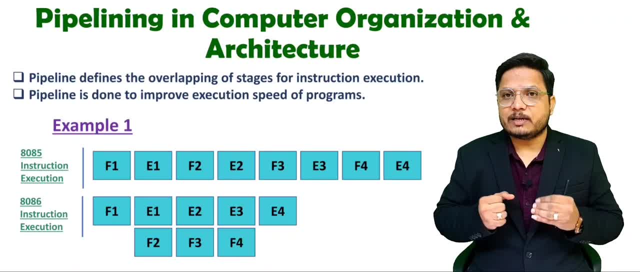 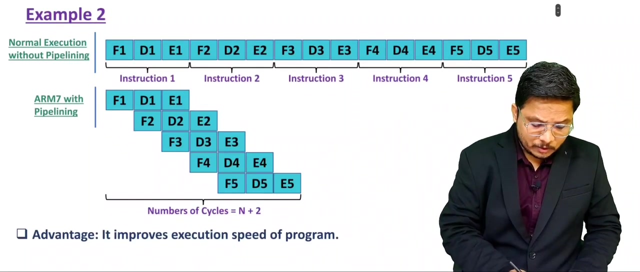 And that is referred as parallel execution of instruction, Right? So you will be observing, there are various computers that is available with various stages of pipelining. Let me give you one more example, That is the regarding ARM 7 TDMI processor, Right, In that there was three stage pipelining. So if you observe that second example, in that you see without pipelining what is happening, fetch decode- execute. Fetch- decode- execute. 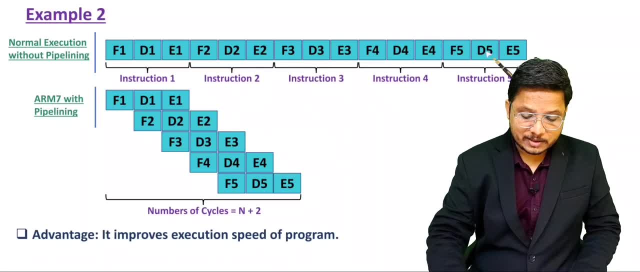 That is how instructions are getting executed And for five instructions you can say at least five into three means 15 clock cycles- that we need to have it to have execution of five instructions. But in ARM 7 TDMI we are having three stage pipelining In that you see first instruction that is getting fetched over here in first clock cycle and in second cycle when it is getting decoded. in that parallel you will be observing second instruction that is getting fetched. 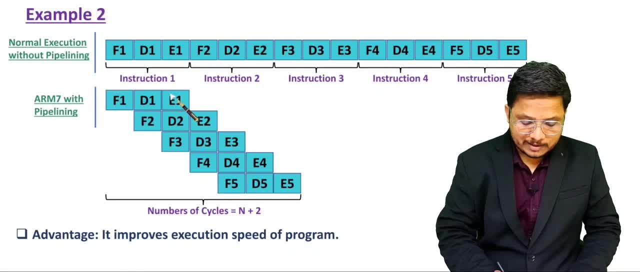 Right, And in third clock cycle, first is getting executed in parallel with that, second is getting decoded and third is getting fetched. When second is getting executed in parallel with that, third is getting decoded and fourth is getting fetched. When third is getting executed in parallel with that, fourth is getting decoded and fifth is getting fetched. And that is how, in parallel, execution of instruction is happening. So if you observe how many clock cycles that we need to have over here, number of instructions. 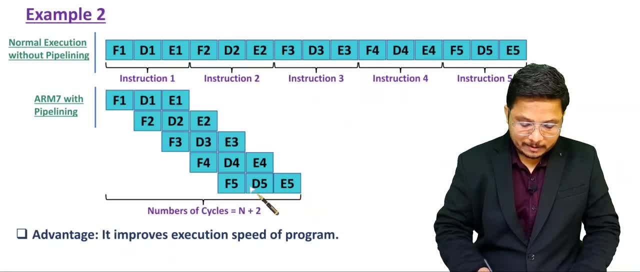 Plus two. you see here five instructions are there, Right? So how many clock cycles that we need to have first, second, third, four, fifth, sixth and seven. So for five, instruction execution with three stage pipelining, you need to have number of instruction plus two means for five, you need to have seven cycles of execution, while without pipelining it was taking five into three means 15 clock cycles. So here, basic, fundamental is what my dear students, 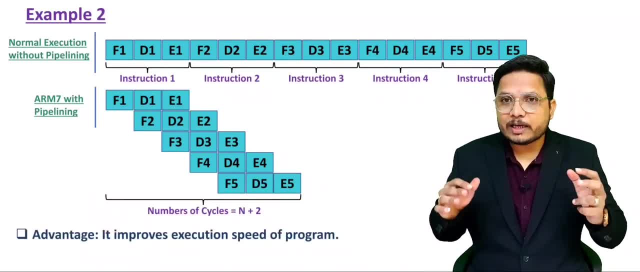 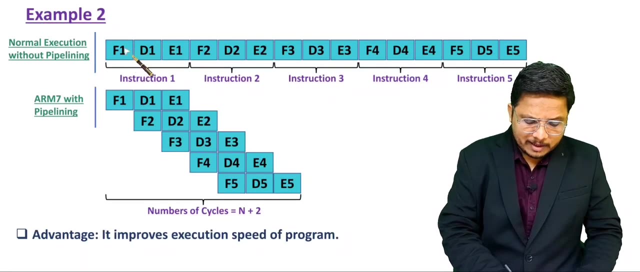 Basic, fundamental is here we are keeping all the units of CPU busy and because of all the units are busy, parallelly execution is happening. and because of parallel execution is happening, entire speed that is getting boosted over here. Like you see here, when first instruction is getting fetched, second is getting decoded over here, Right, And second is getting fetched over here. So you see when fetch is happening, at that time decode and execute. those units are free. 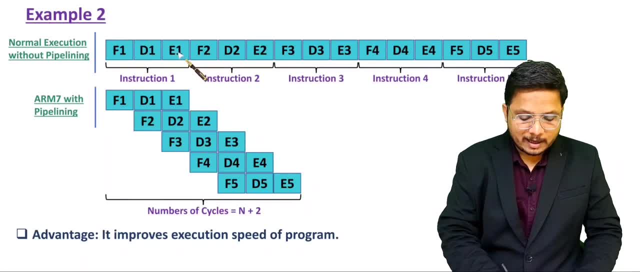 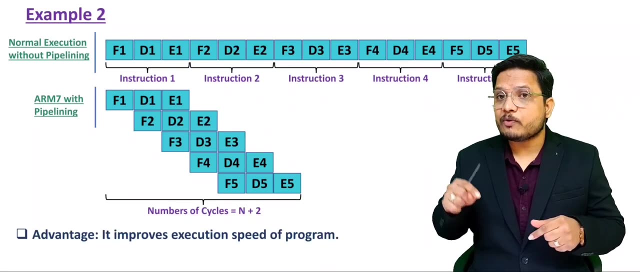 When decode is happening, at that time fetch and execute units are free. When first is getting executed, at that time fetch and decode unit, those are free. And because of sequential execution of all those micro operations, you will be observing only one unit. that will be busy. But instead of that, if you go for pipelining, then what will happen in pipelining, you will be keeping all the units as busy. Now there are a few more basics that I would like to inform you. Like see it is. 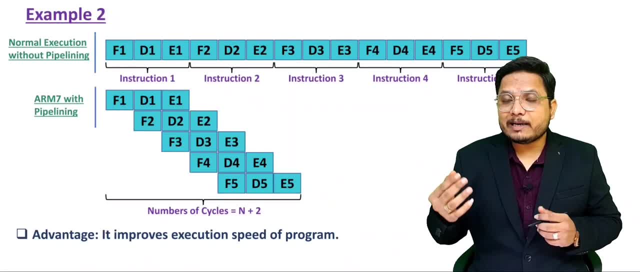 not about only two stage pipelining or three stage pipelining In market. there are many computers that is having various formats of pipelining, Like as if you see ARM 9 processor. in that you will be observing there is five stage pipelining. Right In that stages will be as per fetch, decode, execute memory and write back Right. Likewise, there are various computers that is having multi stage pipelining, Like as if you see Pentium processor in that.